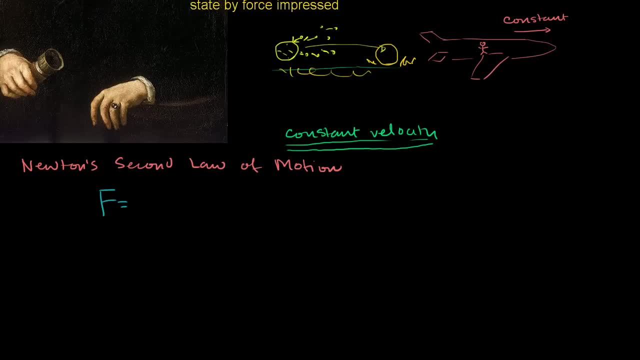 But this one gives us the famous formula: Force is equal to mass times, acceleration, And acceleration is a vector quantity And force is a vector quantity. And what it tells us? because we're saying, OK, if you apply force it might change that constant velocity. 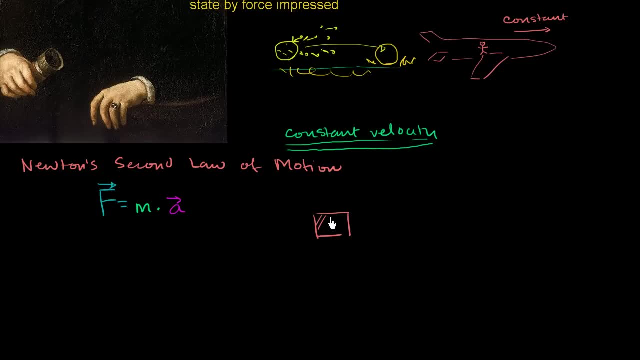 But how does it change that constant velocity? Well, say, I have a brick right here And it is floating in space. Newton's second law tells us that it's pretty nice for us that the laws of the universe, or at least in the classical sense, before Einstein showed up. 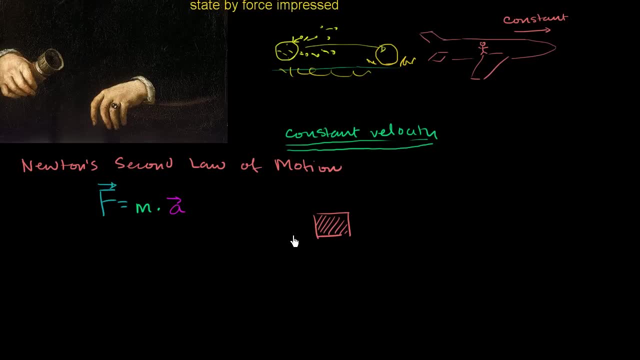 the laws in the universe actually dealt with pretty simple mathematics. What it tells us is if you apply a net force, let's say on this side of the object- And we talk about net force because if you apply two forces that cancel out and then have zero net force. 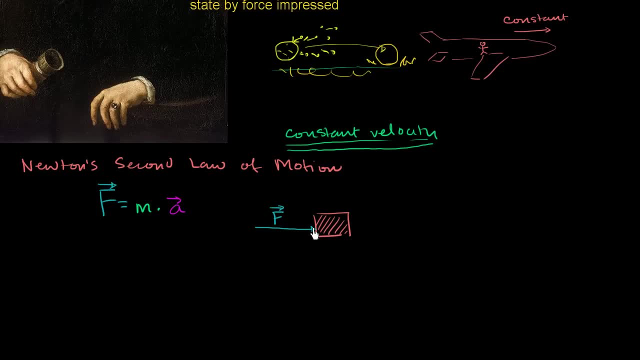 then the object won't change its constant velocity, But you need it. So if you have a net force applied to one side of this object, then you're going to have a net acceleration going in the same direction. So you're going to have a net acceleration going. 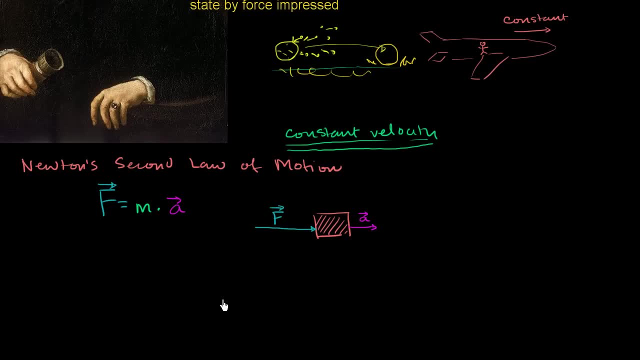 in that same direction And what Newton's second law of motion tells us is that acceleration is proportional to the force applied, or the force applied is proportional to that acceleration. And the constant of proportionality. or to figure out what you have to multiply the acceleration. 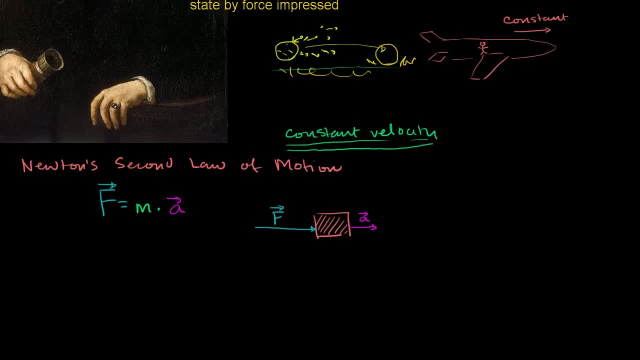 by to get the force, or what you have to divide the force by to get the acceleration is called mass, And I'll make a whole video on this. You should not confuse mass with weight, And I'll make a whole video on the difference. 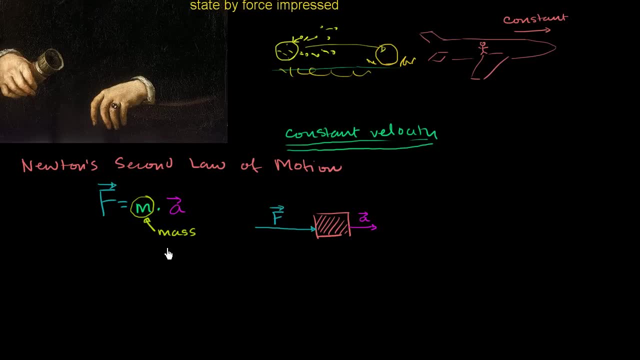 between mass and weight. Mass is a measure of how much stuff there is Now that we'll see in the future. There are other things that we don't normally consider, stuff that does start to have mass, But for our classical- or at least a first year- physics. 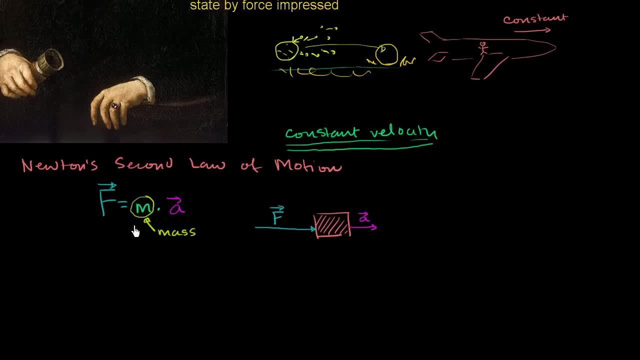 course you could really just imagine how much stuff there is. Weight, As we'll see in a future video, is how much that stuff is being pulled down by the force of gravity. So weight is a force. Mass is telling you how much stuff there is. 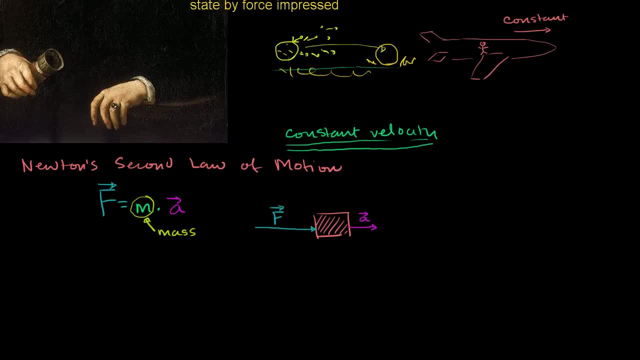 And this is really neat, that this formula is so simple, Because maybe we could have lived in a universe where force is equal to mass squared times- acceleration times, the square root of acceleration, which would have made all of our math much more complicated, But it's nice. 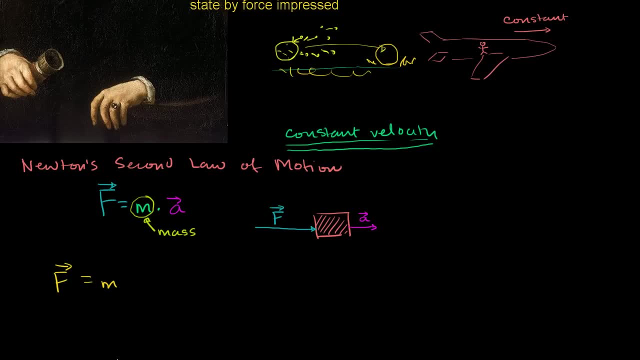 It's just this constant of proportionality right over here. It's just this nice, simple expression. And just to get our feet wet a little bit with computations involving force, mass and acceleration, let's say that I have a force And the unit of force is appropriately. 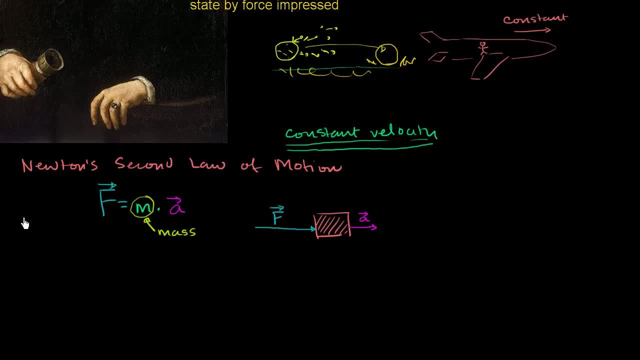 called the Newton. So let's say I have a force of 10 Newtons And just to be clear, a Newton is the same thing. So this is the same thing as 10. Kilogram meters per second squared. And that's good, that a Newton is the same thing. 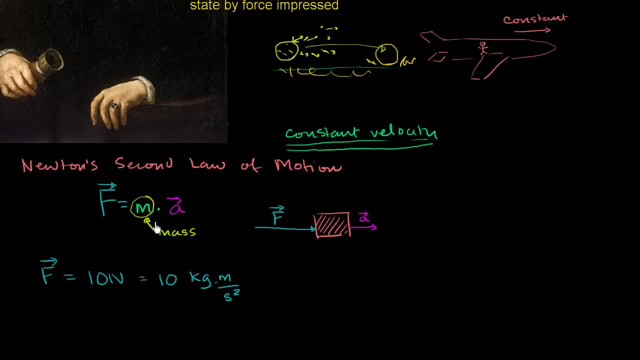 as kilogram meters per second squared, Because that's exactly what you get on this side of the formula. So let's say I have a force of 10 Newtons And it is acting on a mass. Let's say that the mass is 2 kilograms. 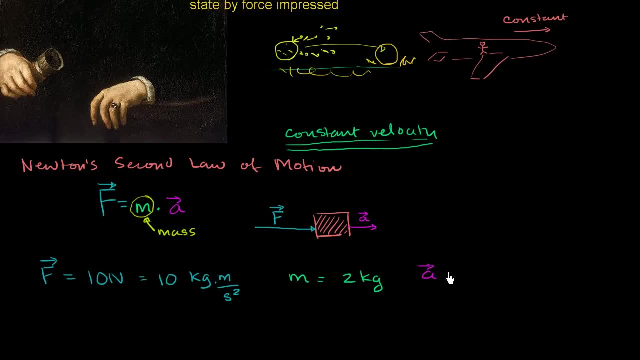 And I want to know the acceleration. And once again in this video, these are vector quantities. If I have a positive value here, we're going to make the assumption that it's going to the right. If I had a negative value, then it would be going to the left. 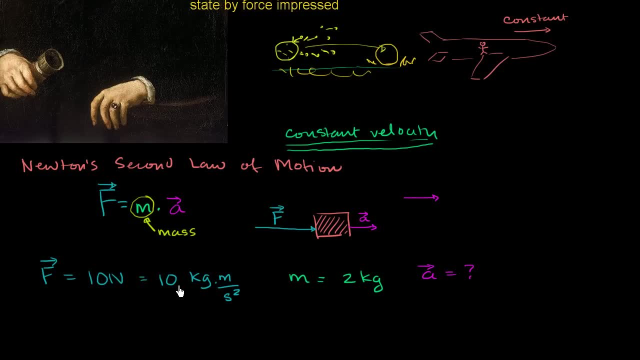 So, implicitly, I'm giving you not only the magnitude of the force, but I'm also giving you the direction. I'm saying it is to the right because it is positive. So what would be the acceleration? Well, we just use F, equals ma. 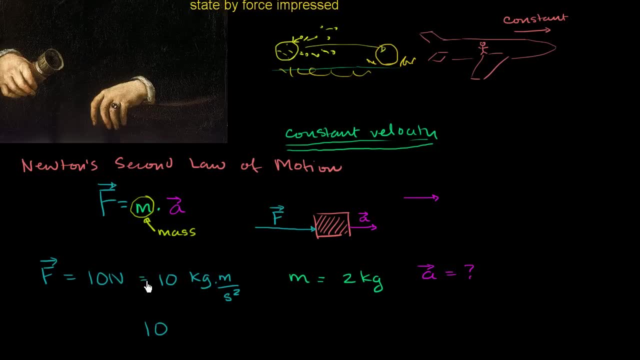 You have on the left-hand side 10.. I could write 10 Newtons here, Or I could write 10 kilogram meters per second squared, And that is going to be 10.. So that's going to be equal to the mass, which is 2 kilograms. 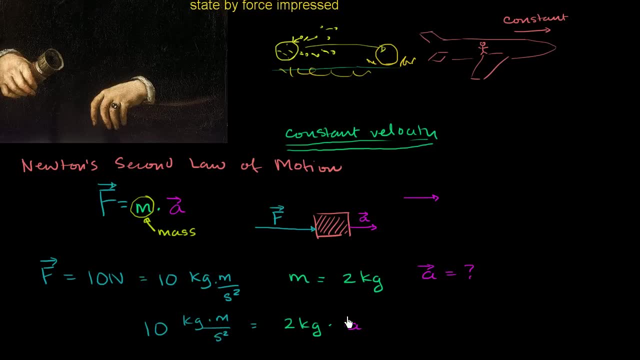 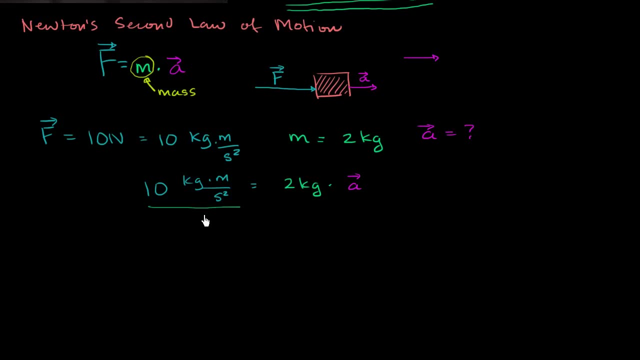 times the acceleration. And then to solve for the acceleration, you just divide both sides by 2 kilograms. So let's divide the left by 2 kilograms. Let's divide the right by 2 kilograms. That cancels out The 10 and the 2,. 10 divided by 2 is, let me just see that.